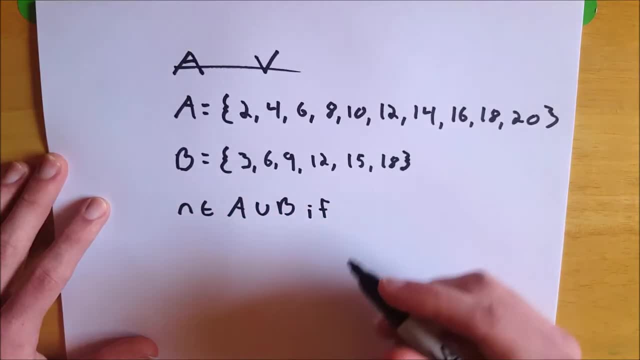 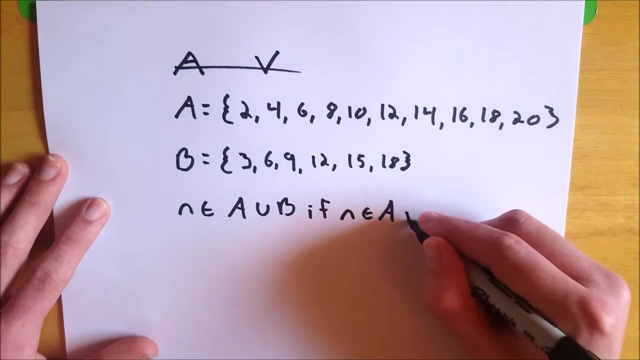 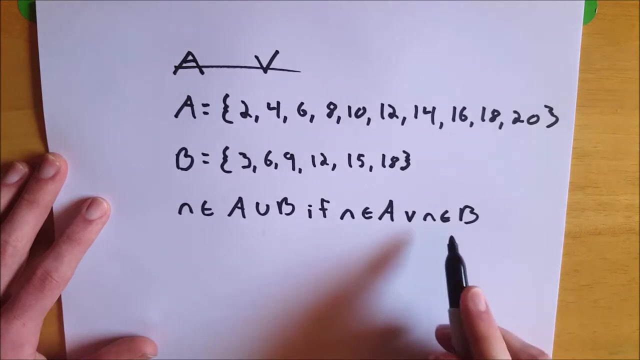 If and only if, but I'm just going to write if, for the sake of convenience. if N is an element of A or N is an element of B, And for those of you who aren't familiar with and or statements, this statement is considered true if this part is fulfilled, if this part is fulfilled or if both parts are fulfilled. 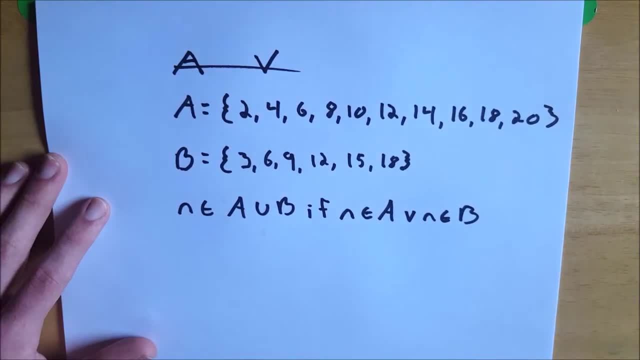 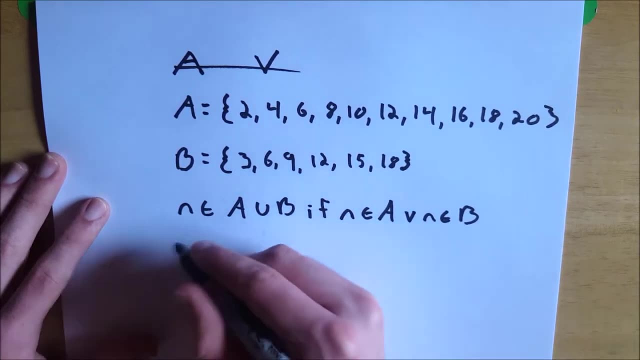 So if N is an element of A, this statement is true. If N is an element of B, This statement is true. If N is an element of A and N is an element of B, then this statement is true, And then N is an element of A intersect B. 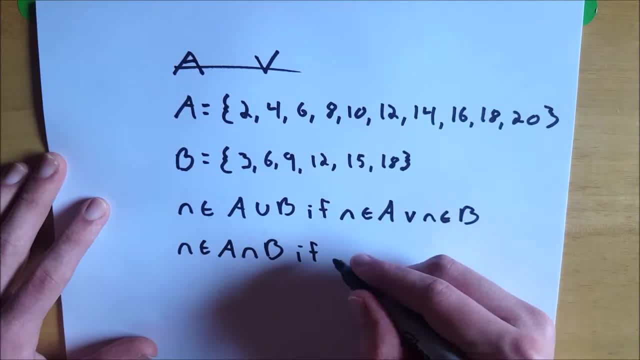 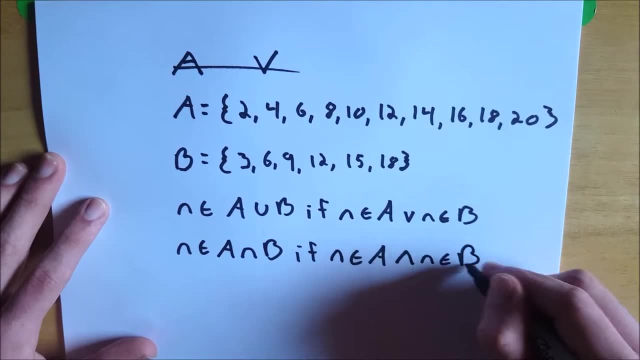 If, and only if- I think there's a short way to write that, but I can't remember off the top of my head. N is an element of A and N is an element of B, So the only time this statement is true is when N is an element of A and N is an element of B. 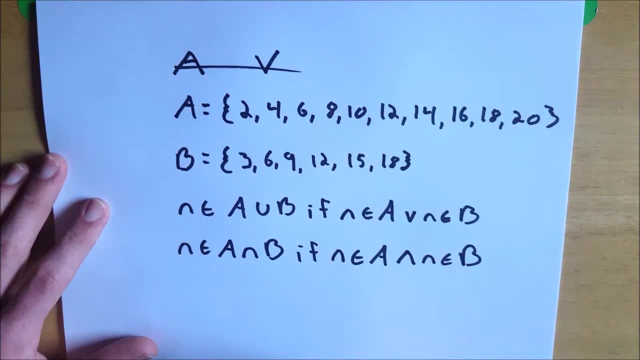 So, with that said, Let's look at A union B and A intersect B directly. you know one after the other, So you really understand this if you struggled after watching the first two videos, or maybe somebody else's videos. So A union B is going to be all the elements that are in A as well as all of the elements that are in B. 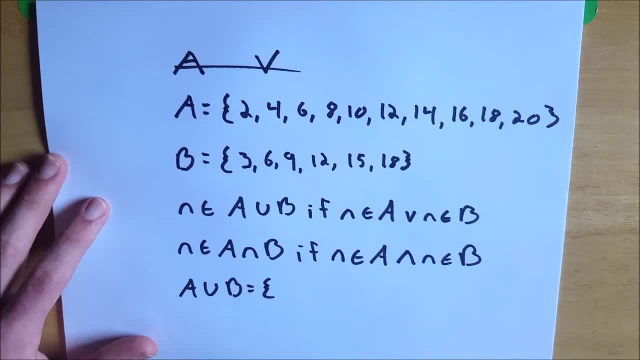 So when you look at a union, you're just putting the two sets entirely together And, as sets go, You're not including any duplicates. So I'm going to write this set out and skip to that. So there's our whole set. A, union B. 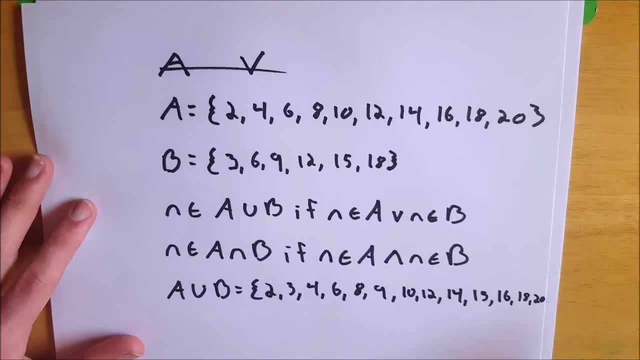 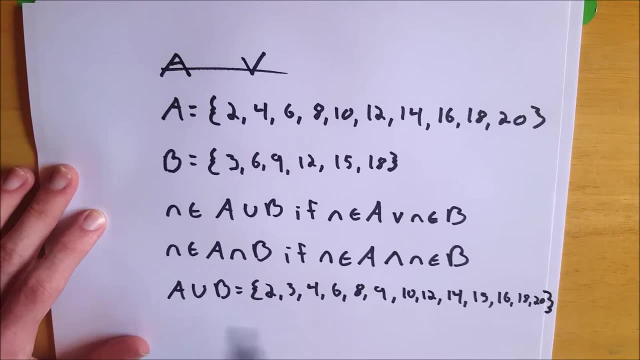 I didn't bother closing it at the end because I didn't have room. Let me slide this paper over and I'll have some room. Yeah, there we go. That's a crappy bracket, but there you have it. That is the whole set. A union B. 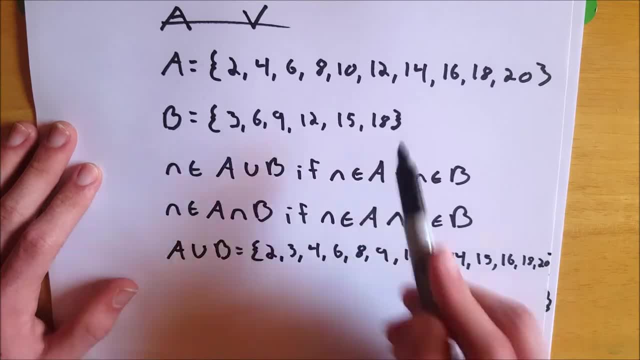 That's all of the elements in A as well as all the elements in B. So every element in this set fulfills this statement That N is an element of A Or N is an element of B. You look at 2, that's in A. 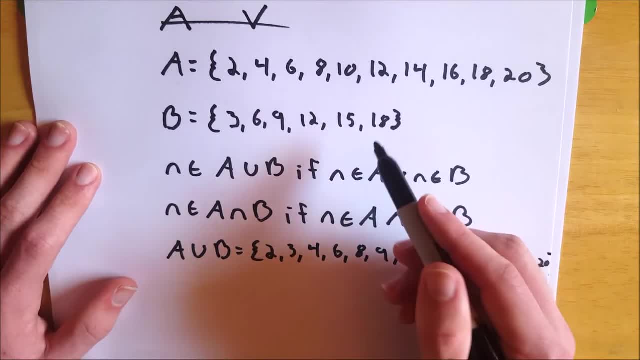 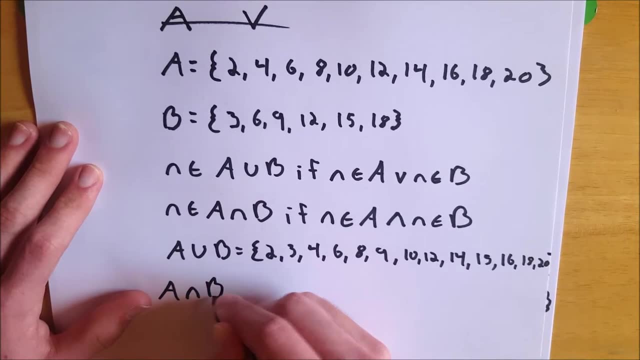 Look at 10,, that's in A, Look at 12,, that's in A and it's in B. So you see how that works. And now let's look at A intersect B. Now, this one is the one that follows this statement. 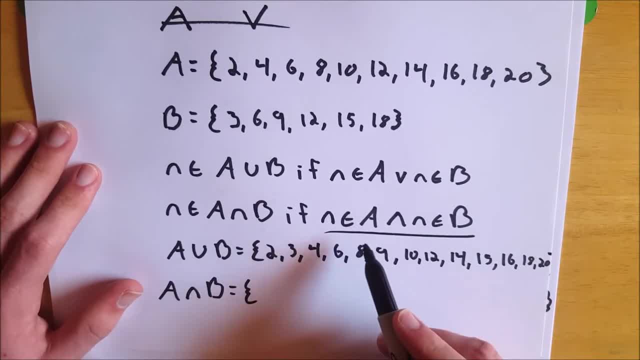 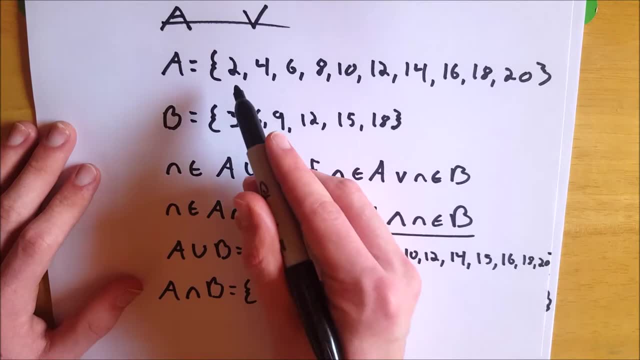 N is an element of A intersect B if, and only if, N is an element of A and N is an element of B. So I'll walk through this one with you because it shouldn't be as long. So is 2 in this set. 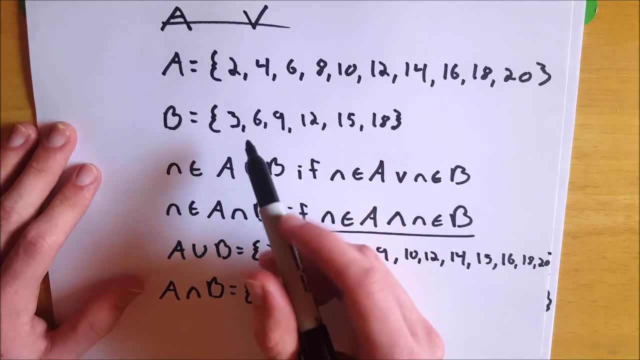 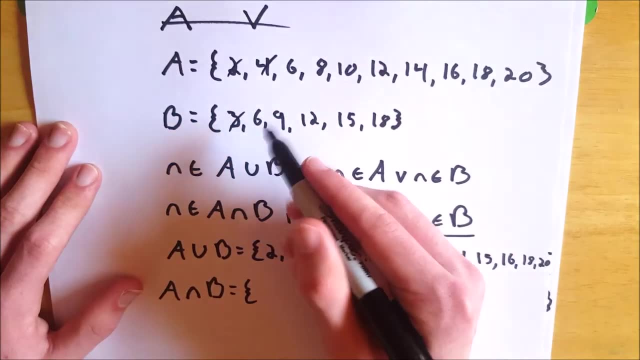 No, it's not, because it's not in B. What about 3?? No, because it's not in A. I'll just cross these off. 4 is not in B, so we can't include that. 6 is in B and is in A. 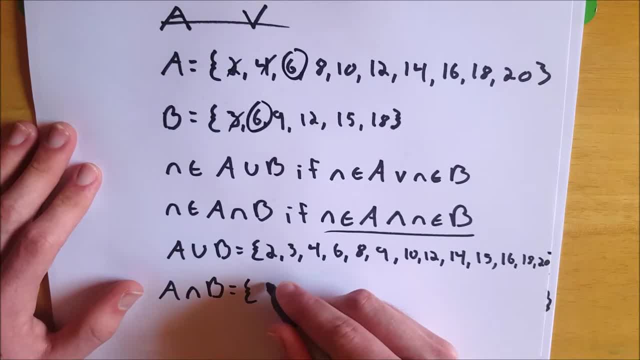 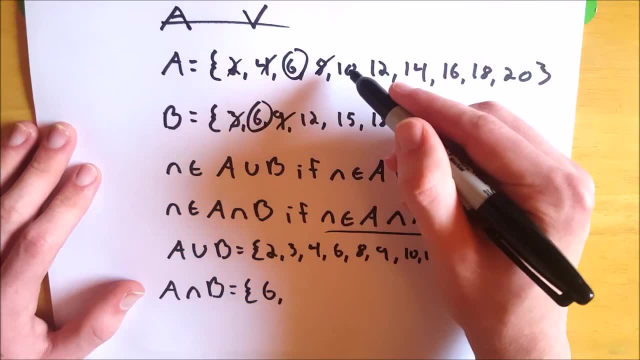 So that's going to be the first element to go into A intersect B. 8 is not in B, 9 is not in A, 10 is not in B, And then 12 is in both of these sets, So it will be in B. 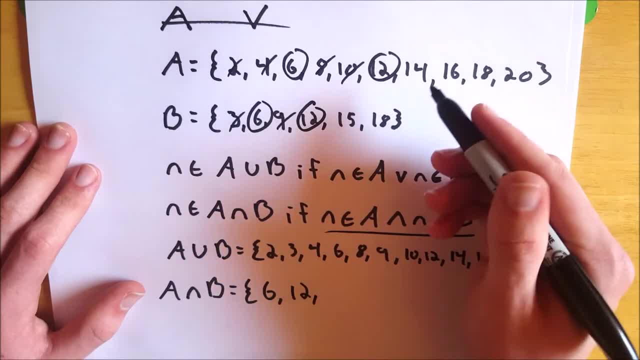 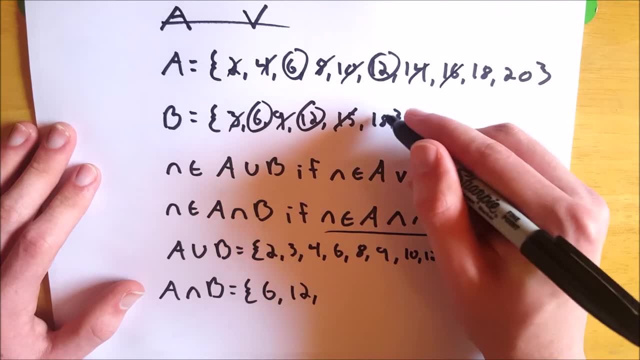 And then 12 is in B, 15 is not in A, 14 is not in B, 16 is not in B, 18 is in both of them. So that will be the next one in our set. And then 20 is not in B. 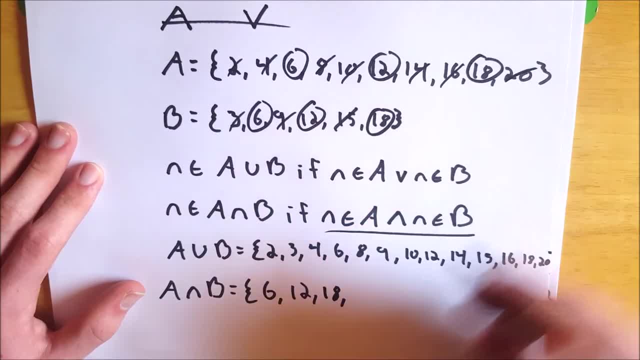 So this is the whole set. A, intersect B. It only has 6,, 12, and 18.. As you can see, it's got all. it has positive multiples of 6.. So it's really just a set of 6.. 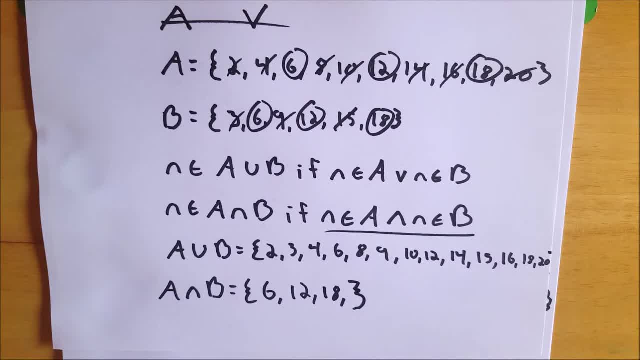 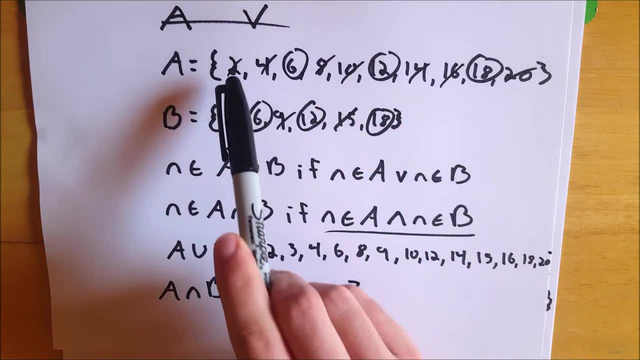 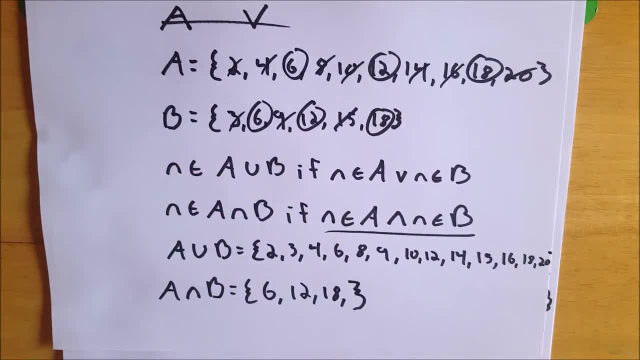 that are multiples of 2 and this set that are multiples of 3.. And that's a hint as far as divisibility rules of 6 go, But I hope that cleared things up. If you're confused about anything else regarding unions and intersections, 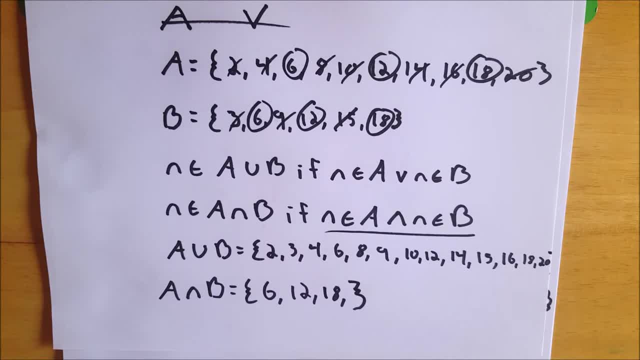 just let me know in the comments, Tell me if there's any other topics you'd like me to cover. But I hope these three videos I've done on unions and intersections have helped explain it to anybody who was unfamiliar with the concepts. So I hope that helped. 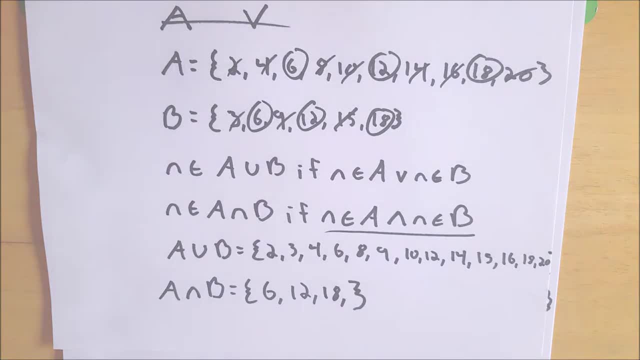 Let me know in the comments. Subscribe for the swankiest math videos on the internet And I'll see you next time.